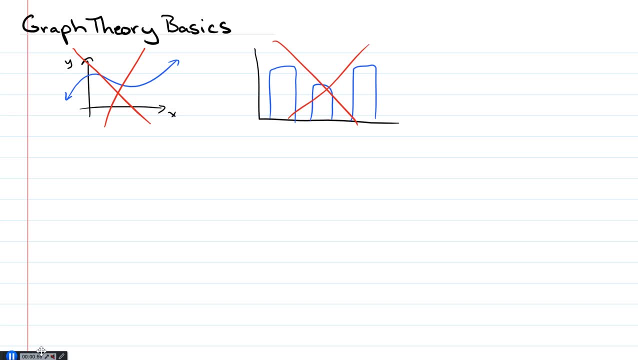 we're talking about. So you might have thought of a graph as something that looks like vertices. That's not what we're talking about with graph theory, And there are all sorts of other graphs. You've got pie charts that well, that's a terrible pie chart, but you get the idea. These are all things that you might. 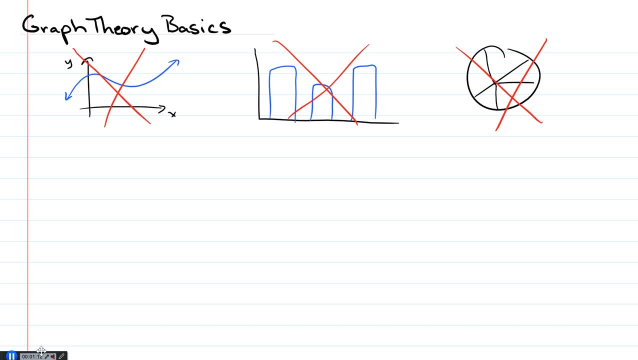 have images of in your head when I say graph, and that's not what we're going to be dealing with here. So wipe all of that away and we're going to start over fresh with this whole new idea of a mathematical graph. And you've got a definition of a graph in your textbook, so I'm not going to. 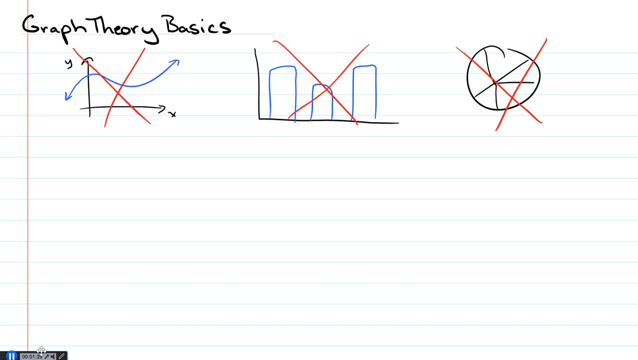 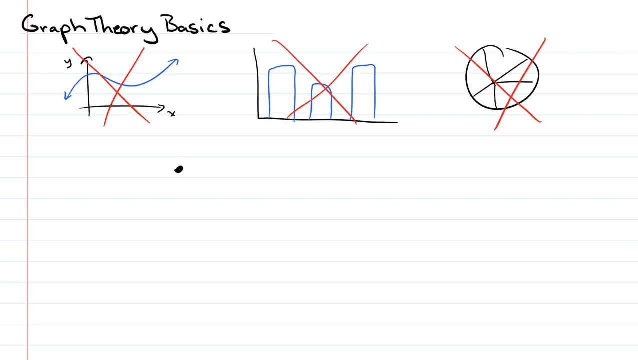 repeat the definition or write the definition down. I'm just going to go through what a graph is. So what a graph is is a collection of these dots. I'll draw some dots here. What these dots are called are vertices. So I have a group of these dots. They're called vertices. 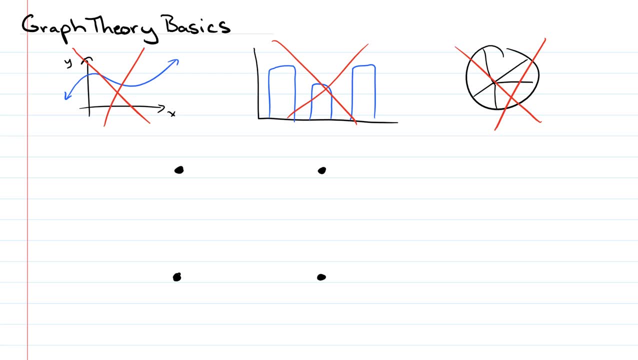 If I just have one dot, by itself, it's called a vertex. All right, you would drive your math teacher nuts if you call one of these a vertices. So make sure that if you're talking about just one of the dots, you're talking about a vertex, and if you're talking about all of the dots, you're. 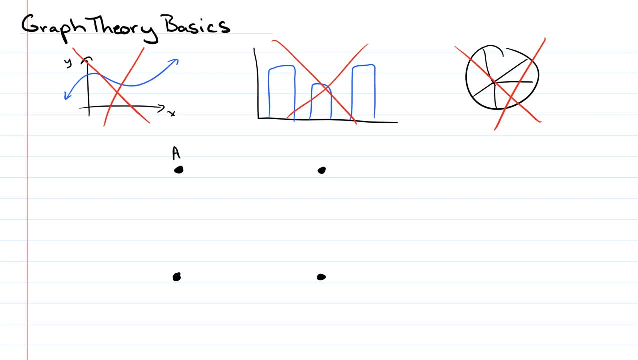 talking about vertices, And I'm going to just give these names. I'll call them A, B, C and D, so that I can keep track of what I'm doing here. And then the other thing that we have in a graph are edges- Edges that connect the vertices, And so I could draw a straight line between A and B. 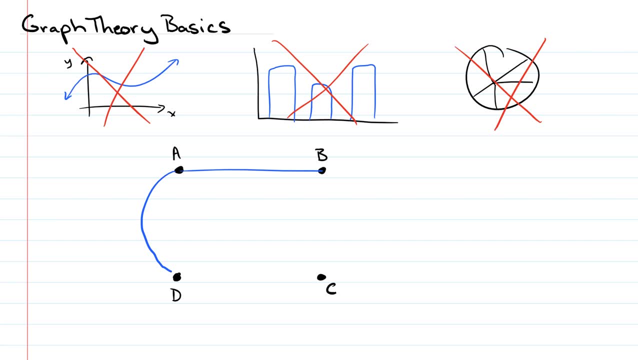 and that would be an edge. I could draw a curved line between A and D. that would be an edge. I could draw a line from C all the way back to itself. that is also an edge. So, basically, what a graph is is going to be a collection of vertices and then the edges that 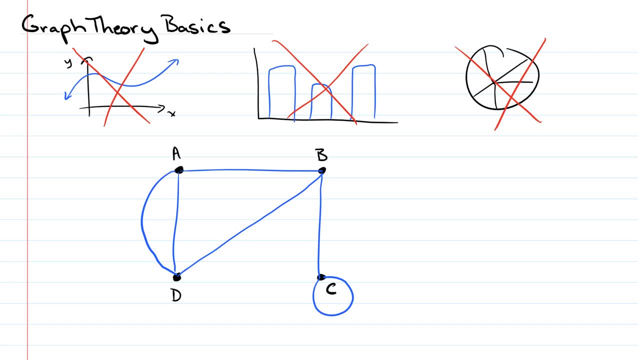 may or may not go between those vertices, And so you can draw a whole bunch of these, and this right here is a graph, So let's label this a little bit here. The dot there, that's a vertex, This right here that is an edge, And this edge here is actually kind of a special edge. It's one. 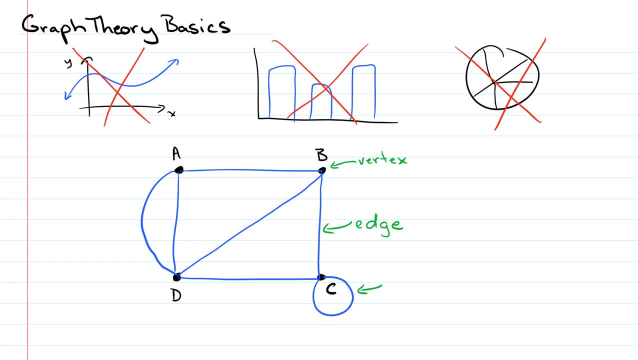 of these things in graph theory where, if you stick with me long enough, you're going to find out there are some special names for a lot of things. The good thing about graph theory is all of these names make a whole lot of sense. So when you've got an edge that goes from a vertex right back to 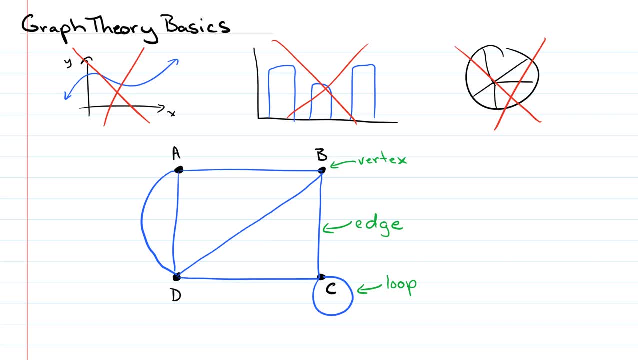 itself. we just call that a loop. All right, so no big deal there. And then I want to make sure that we talk about something that tends to confuse people with graph theory. when they're doing it, first time, They have a good idea about what these vertices and edges are, and then somebody 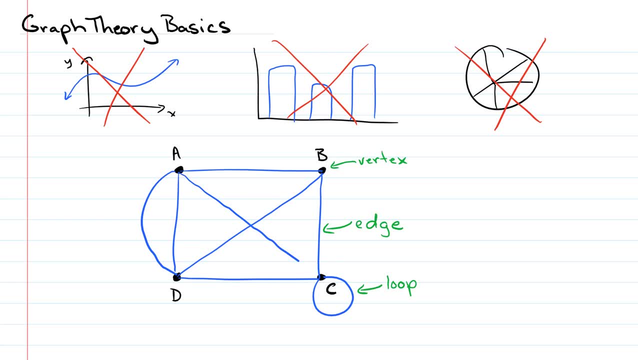 does something like draw an edge between a and c, And so we've got something happening in this area right here. right, It sure looks like those lines are crossing each other, And a big mistake that people make is assuming that this space right here is a vertex, and this is not a vertex You might even want to think about. one of those lines is: 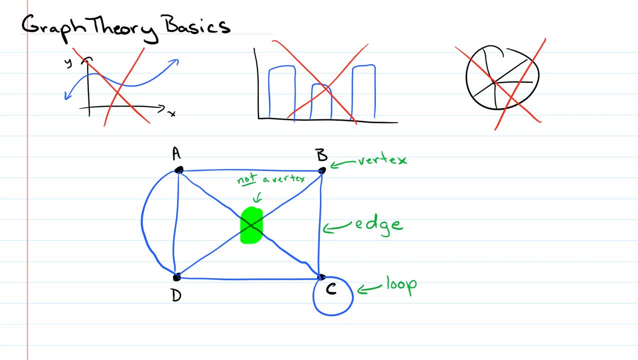 going over and over and over and over again. But that's not going to happen and you might have to the top of the other line, because if they don't actually have a dot drawn on there, that's not a place where those, those two lines actually intersect. so 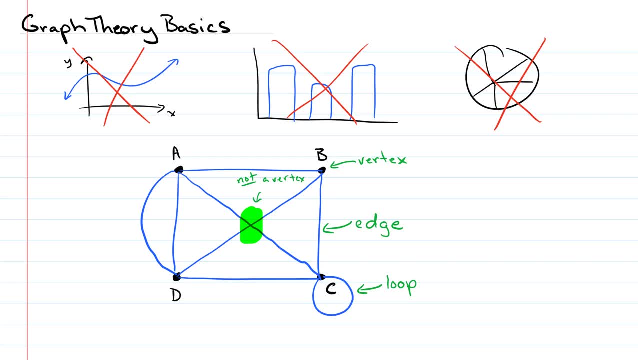 these two lines, the line between A and C and the line between B and D. they don't touch each other at all. so that's not a vertex and that might be something that you see on the test or quiz. at some point somebody might ask you whether or 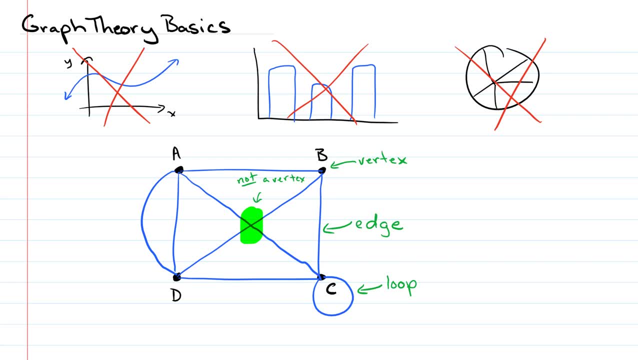 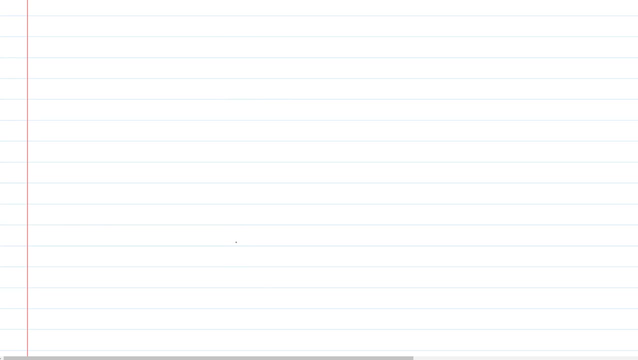 not, there's a vertex in this place and they're just absolutely isn't okay. so let's see what other basic ideas we can talk about. about grass, I'm gonna scroll down a little bit here and we'll talk about equivalent graphs. so equivalent graphs are two graphs that are technically the same- equivalent, I think. 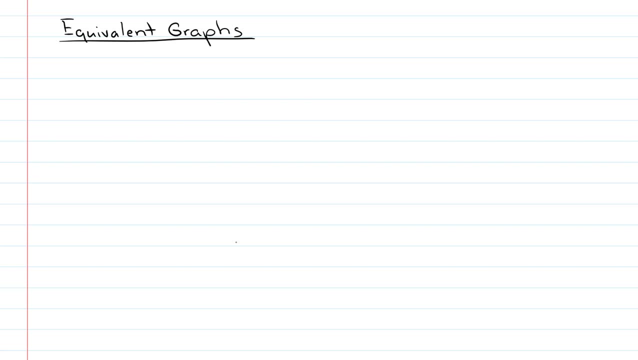 I could spell today. all right. so if I have a set of vertices- my a, a, a, a, a, b, c, d- and I connect them, let's see, I'm gonna do an edge here, an edge here and an edge here. that graph is actually the same as if I just did this, so I'm gonna. 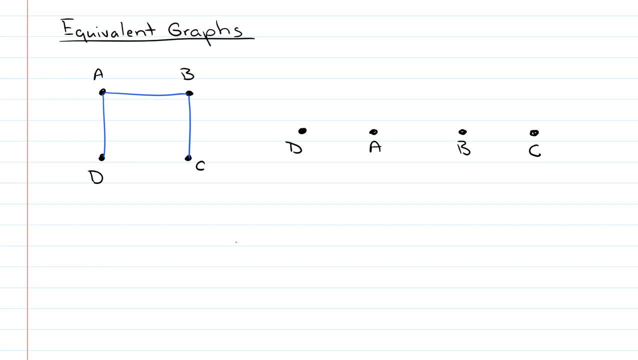 call this D, A, B and C, and I'm going to connect from here to here to here. right? all I did, basically, was flap all the flaps out and call it the same thing. so two graphs are equivalent when they've got the same number of vertices and the 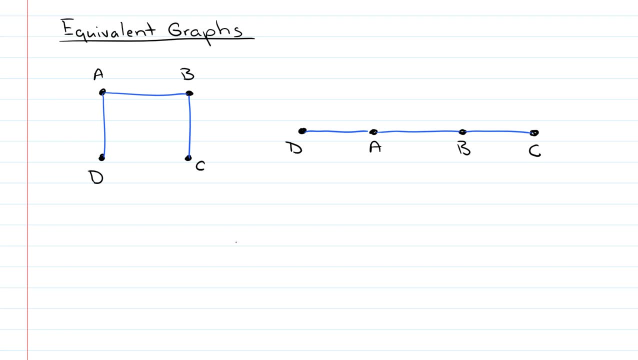 same edges between those specific vertices. so here I've got an edge between A and D. here I've got an edge between A and D. here I've got an edge between A and B. got an edge between A and B. I've got an edge between B and C. here I've got an edge. 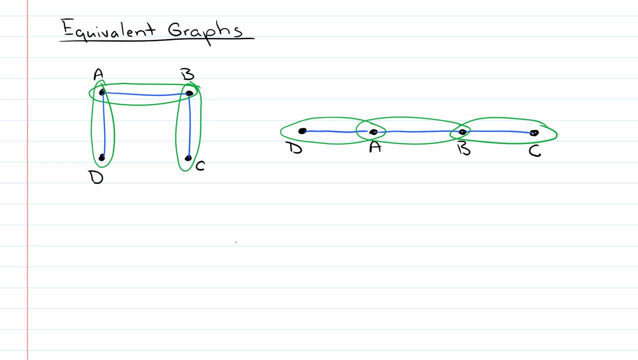 between B and C. so same number of vertices, same number of edges, and the edges go between the same vertices. so it can be a little weird sometimes because graphs that don't necessarily look alike really are the same thing. so here's one to show you the point of equivalent graphs. so here's an A, B, B. 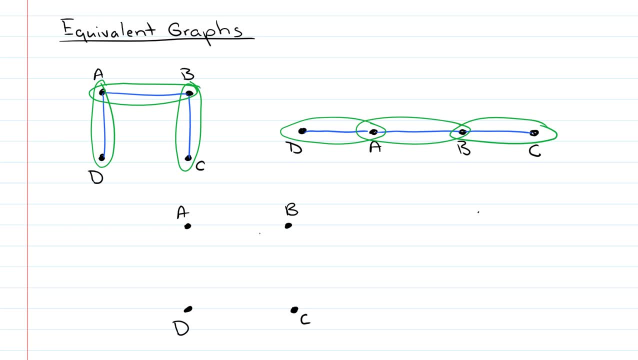 C, D, And then I'm going to draw this A, B, C and D, so call it A, B, C and D. so I'm going to draw an edge here and an edge here, an edge here and edge here and an edge here and an edge here. 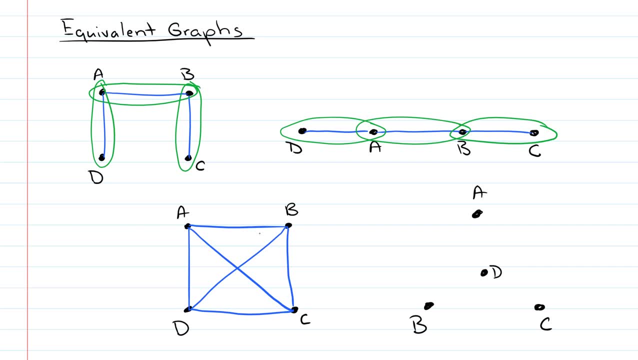 now remember the middle. there there's no vertex. the only vertices we have are A, B, C and D. All right, so I have an edge between A and B, so I'm going to draw one between A and B. Well, it looks like I've also got one between A and C, so I'm going to draw an edge between. 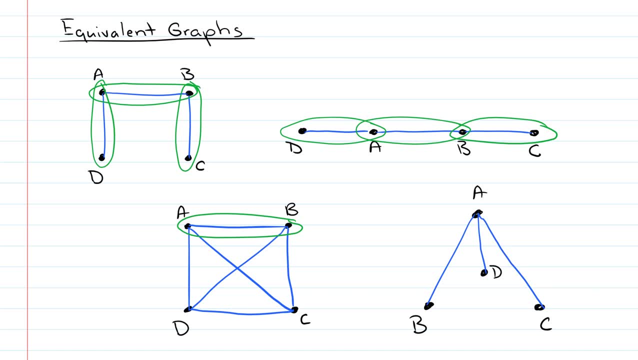 A and C. I have an edge between A and D, so I'll draw an edge between A and D And I'm going to stop circling those because it's going to get pretty crowded there in a second, So I'm going to move on to B. I've got an edge between B and A. I've already drawn that. 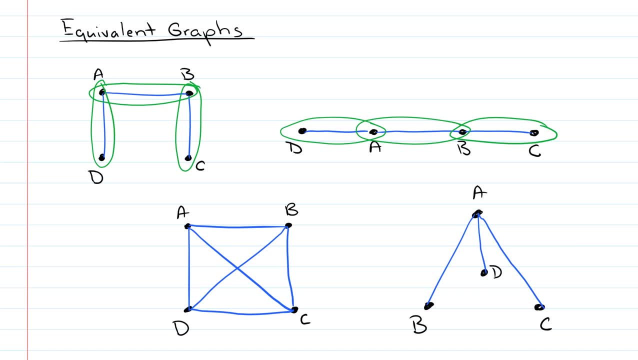 I've got an edge between B and C, so I'll draw that one. Oops, the right color here, And now I need an edge between B and D, so I'll draw that. And now we'll move on to vertex C, C and B I've already got. 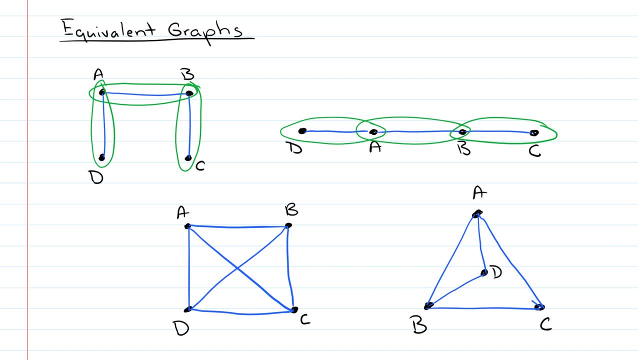 C and A I've already got, so I need C and D. I have an edge between C and D, And now, by the time I make it to D, I've got all of the edges that I need. So these two graphs are actually- they're equivalent.